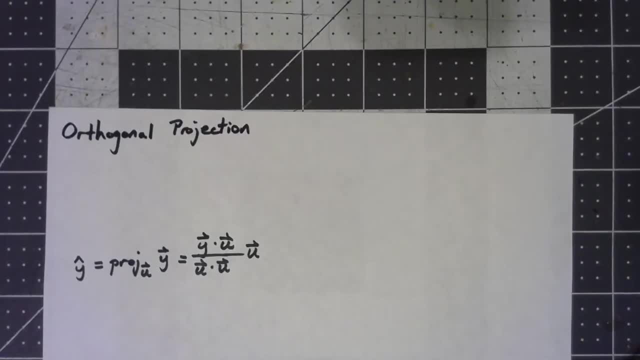 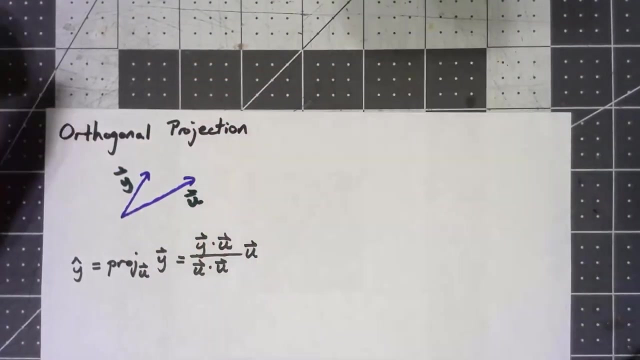 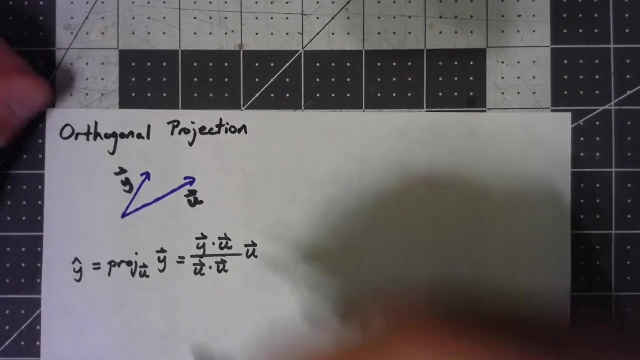 If we have two vectors, we can do what we call projecting one vector onto another. Here's the basic idea. Let's say I have a vector here and a vector here. Let's call this vector y and this vector u. The projection of y onto u is basically saying, if I drop a perpendicular down here: 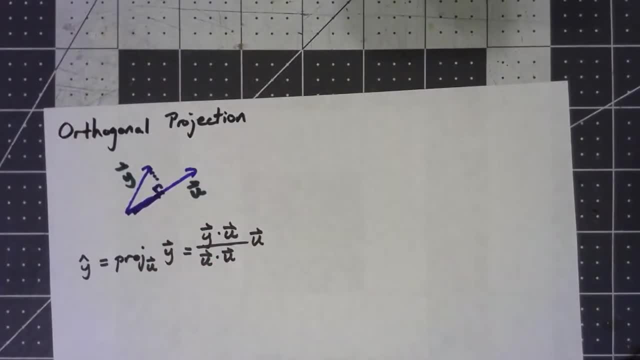 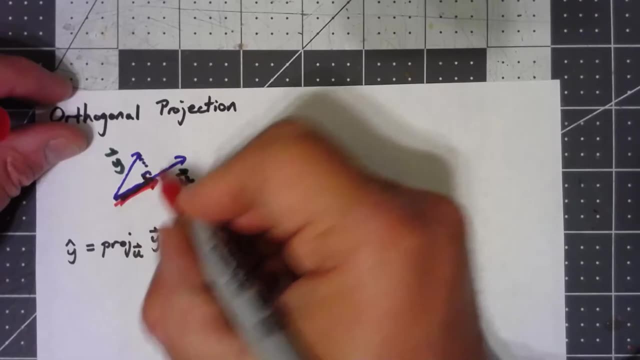 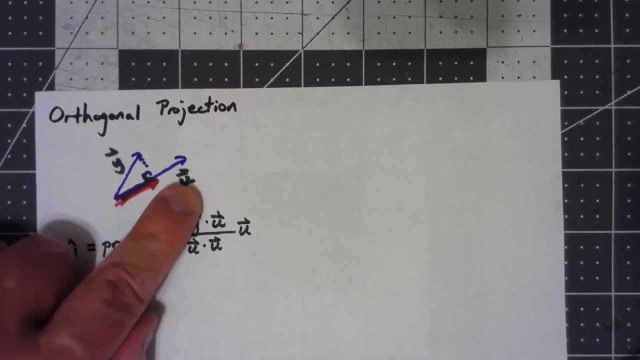 then we get a vector in the same direction as u, but only has a length that goes to there. The basic idea is: you're trying to find the part of the vector y that is perpendicular to u. Now I drew the simplest case here first. but what if I had, for example, a vector u? 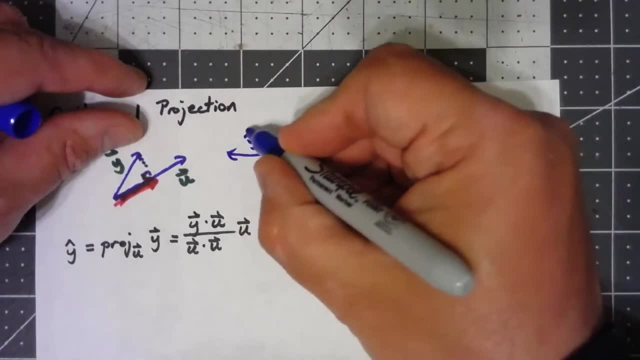 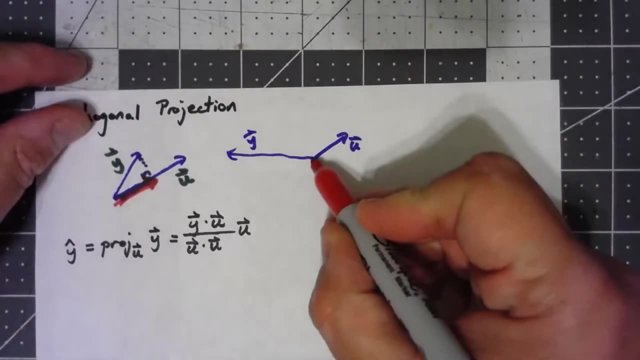 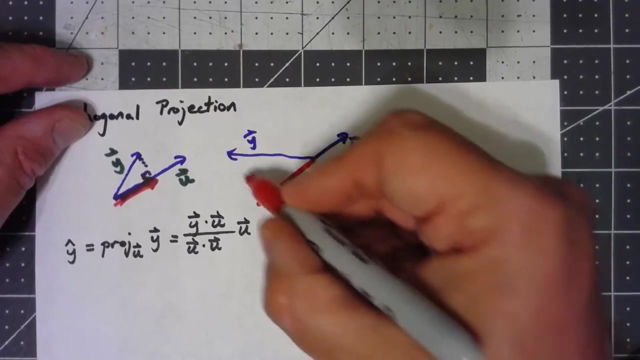 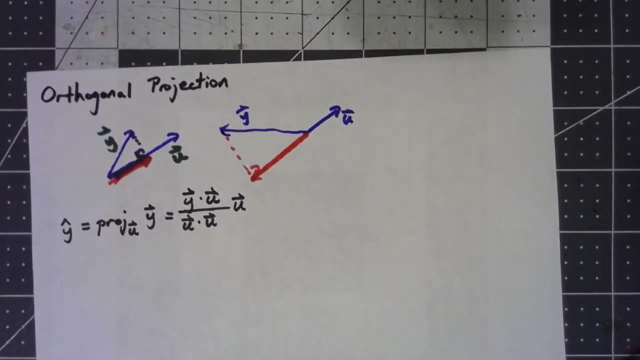 and a vector y was out here. We can still project y onto u, but we kind of get something back this way. instead We sort of extend the u in the opposite direction, go down perpendicular, like that, and so this red vector here is the projection of y onto u. So how can I figure out how this works? Well, the formula's. 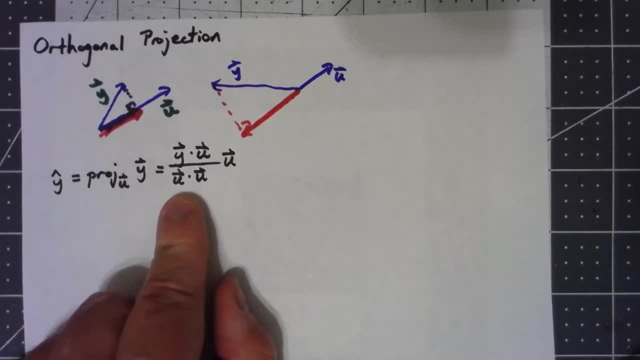 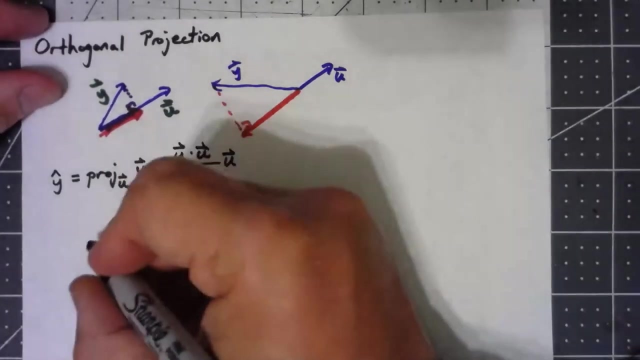 been staring at us this whole time. To figure it out, I take the dot product of y with u over the magnitude of u squared, just u dotted with itself times u vector. So let's do a simple example. If I want to say my y vector is: 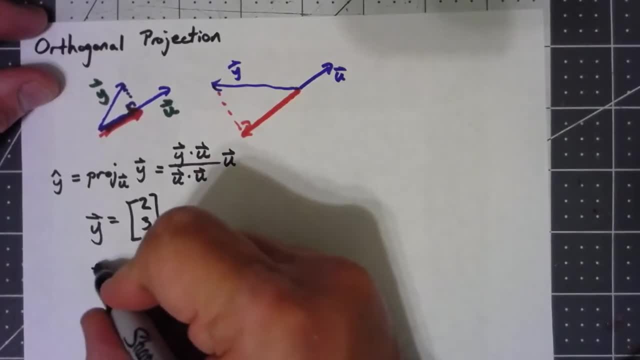 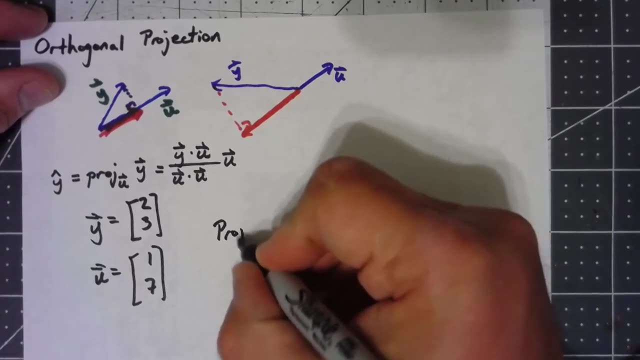 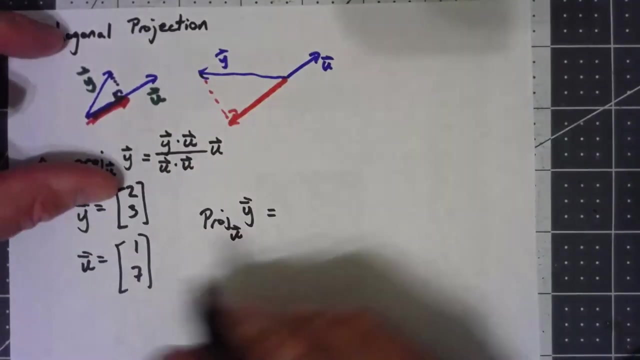 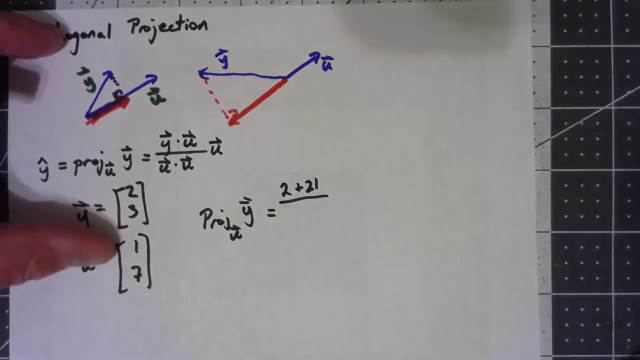 and I want to project that onto a vector u. maybe the projection of vector y onto u is: dot these two things. things would be 2 plus 21 over u. dotted with itself would be 1 plus 49. And then that's times u vector. 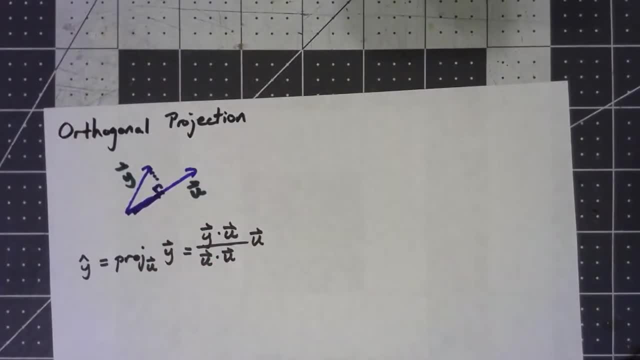 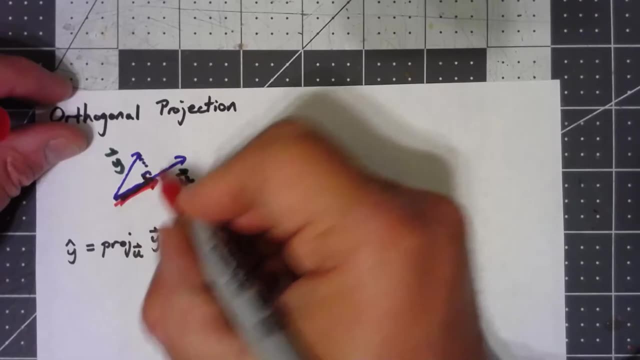 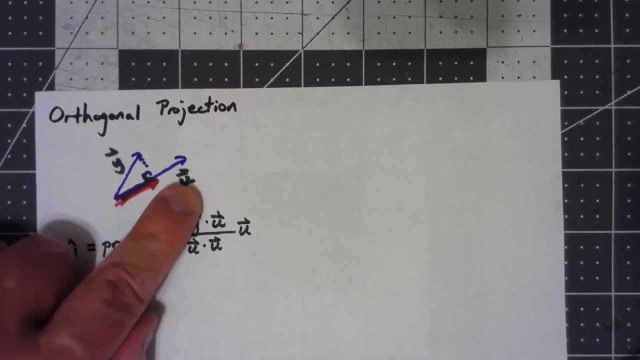 then we get a vector in the same direction as u, but only has a length that goes to there. The basic idea is: you're trying to find the part of the vector y that is perpendicular to u. Now I drew the simplest case here first. but what if I had, for example, a vector u? 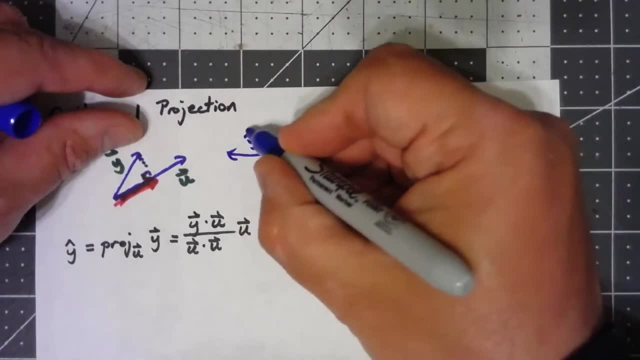 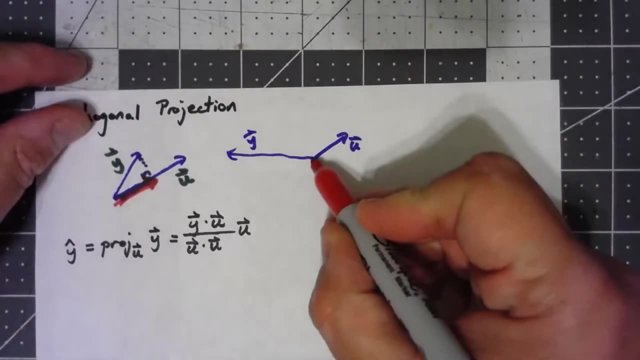 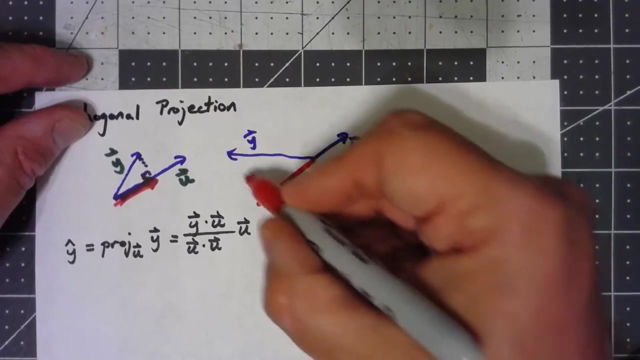 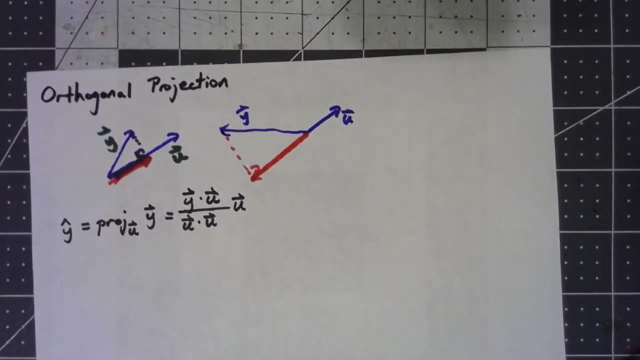 and a vector y was out here. We can still project y onto u, but we kind of get something back this way. instead We sort of extend the u in the opposite direction, go down perpendicular, like that, and so this red vector here is the projection of y onto u. So how can I figure out how this works? Well, the formula's. 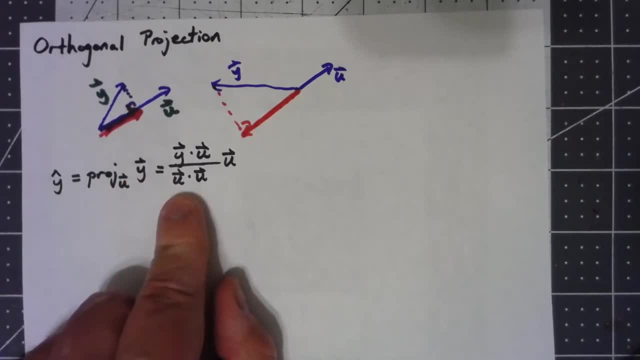 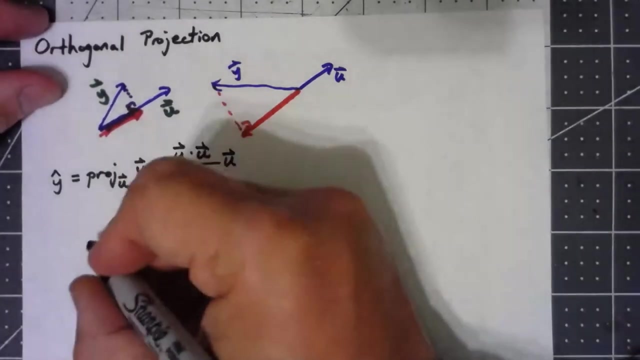 been staring at us this whole time. To figure it out, I take the dot product of y with u over the magnitude of u squared, just u dotted with itself times u vector. So let's do a simple example. If I want to say my y vector is 2,, 3,. 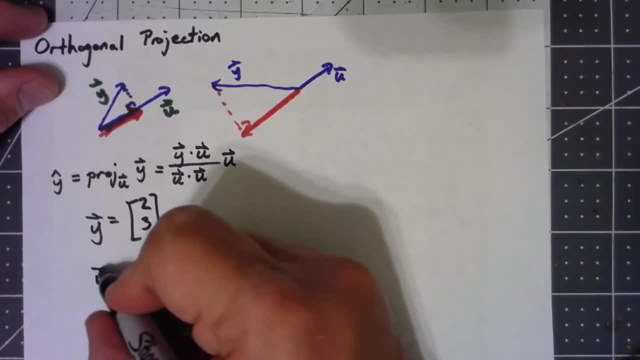 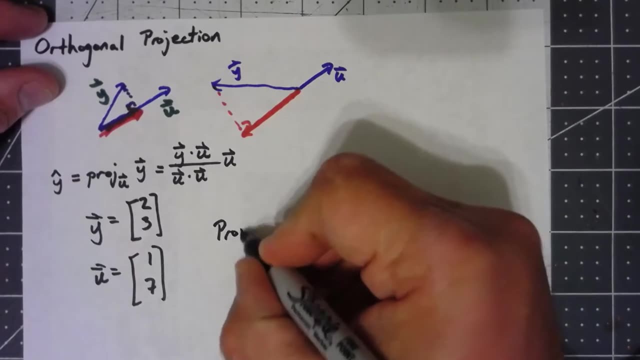 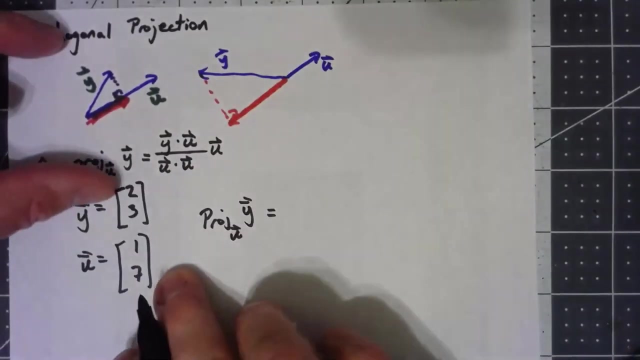 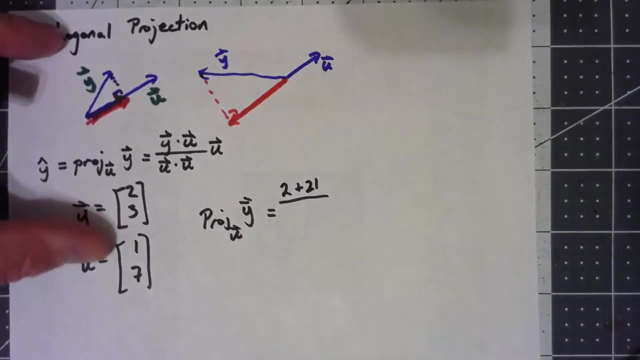 and I want to project that onto a vector u maybe 1, 7,. the projection of vector y onto u is: dot these two things. two things would be 2 plus 21 over u. dotted with itself would be 1 plus 49,. 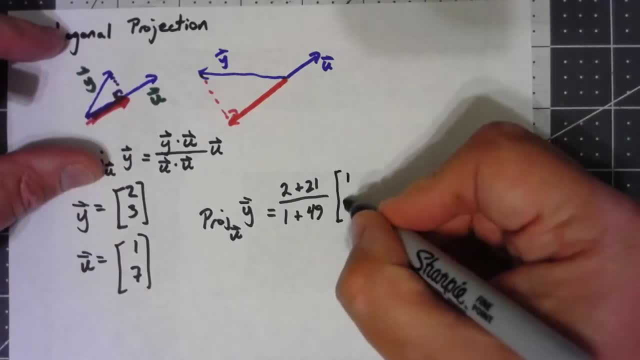 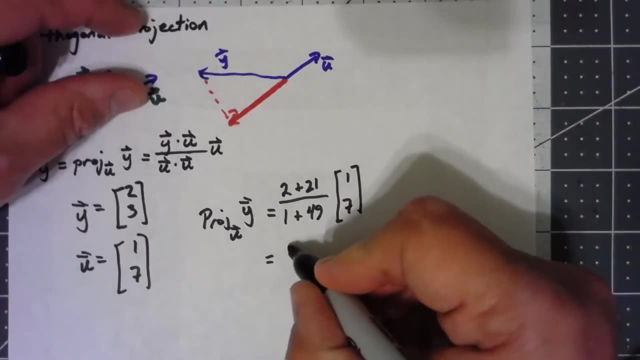 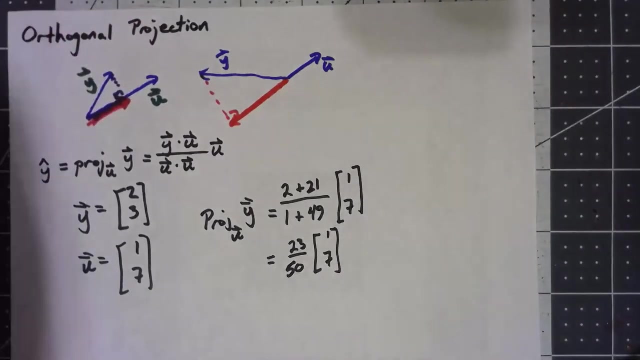 and then that's times u vector, That's times the vector 1, 7.. So I've got 23 50ths times 1, 7, and I'm just going to leave it like that. Certainly we could distribute the 23 50ths times that. Now, another thing that's worth noting about. 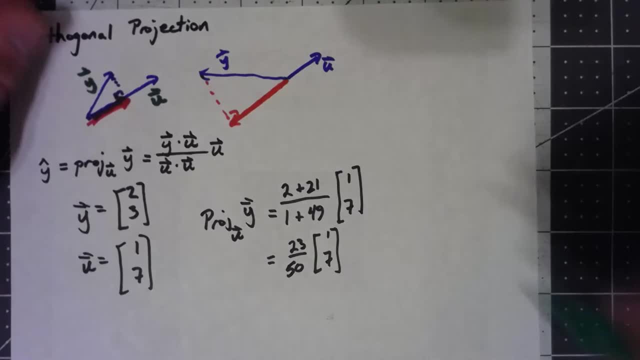 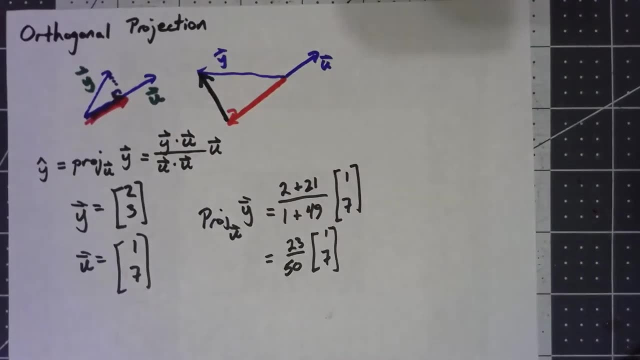 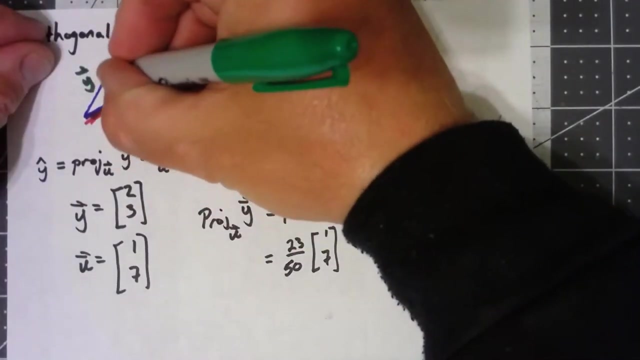 this is that. what is this vector here? Well, it's actually very simple. Well, it's actually very simple. Well, it's actually very simple. That vector there, in either case, it'd be this one here. that vector is y minus that projection. 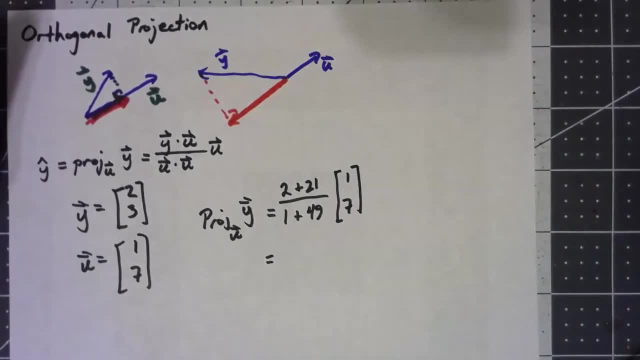 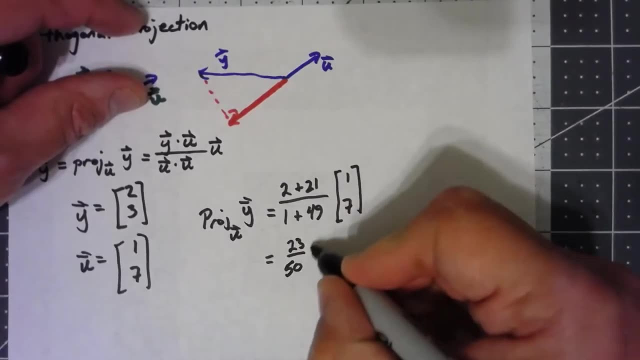 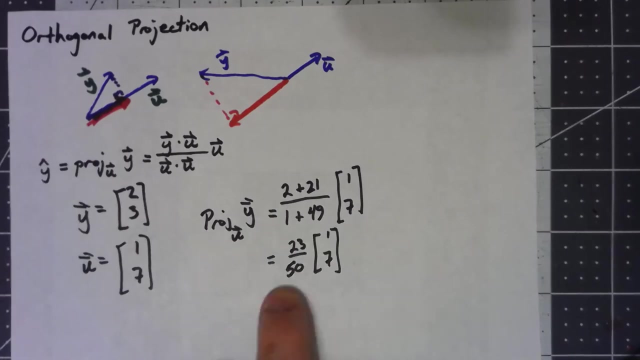 That's times the vector 1, 7.. So I've got 23 50ths times 1, 7. And I'm just going to leave it like that. Certainly, we could distribute the 23 50ths times that. 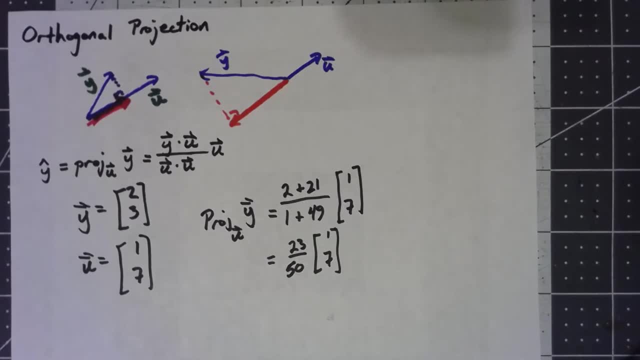 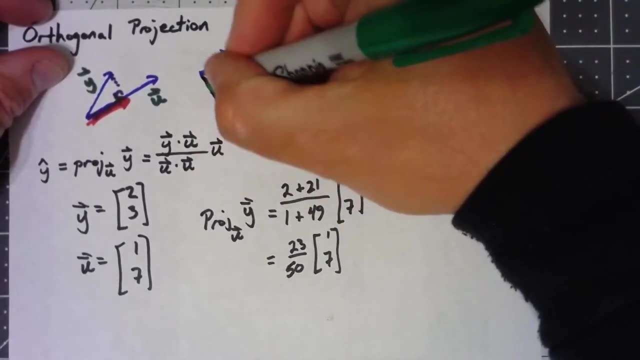 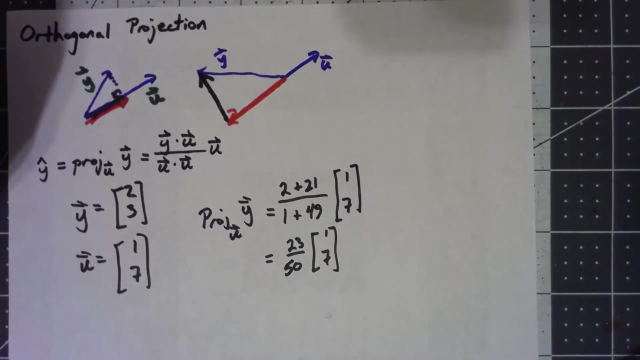 Now, another thing that's worth noting about this is that what is this vector here? Well, it's actually very simple. That vector there, in either case, it would be this one here. that vector is y minus that projection. The whole idea is that this red vector plus this green vector. 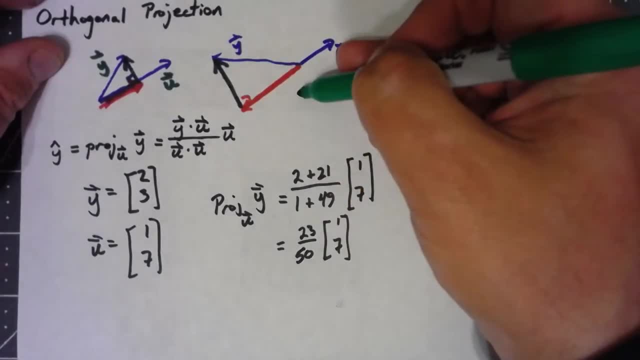 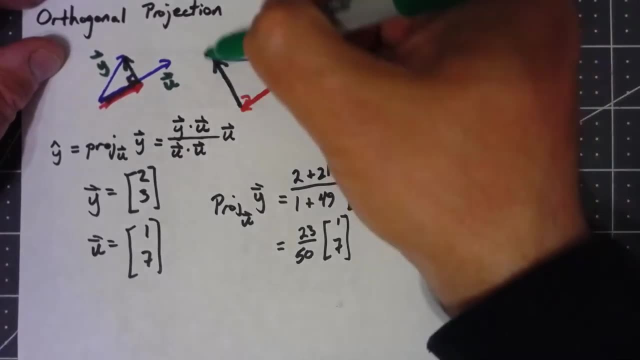 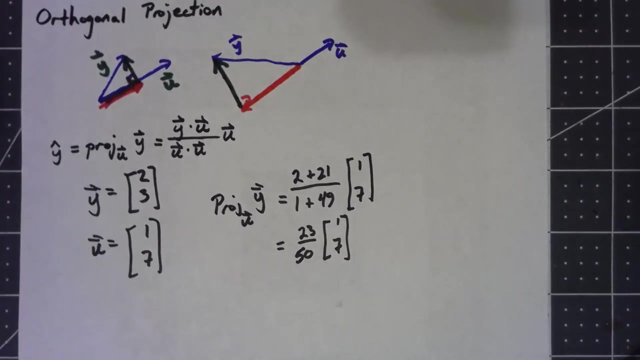 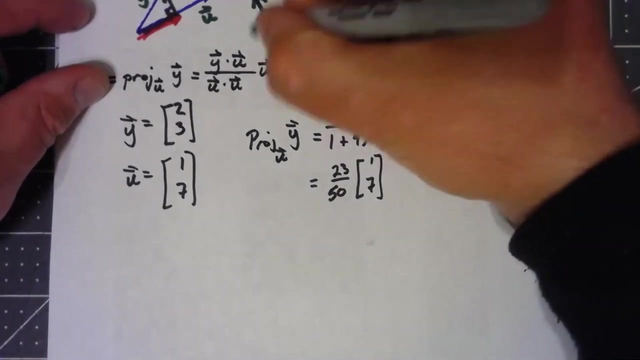 has to be equal to y and further the red part of it. the projection is parallel to u, whereas the green portion is perpendicular to u. So, like I said, it's because those two parts have to add up to y. let's call this thing y. 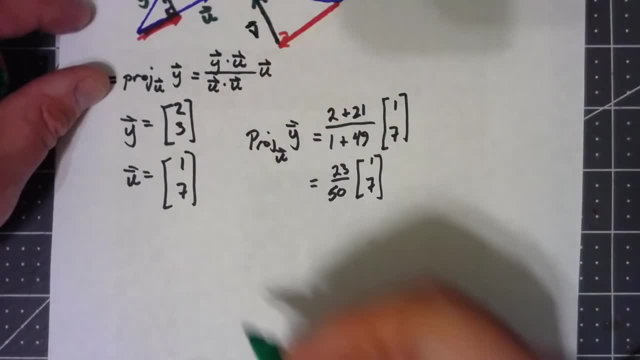 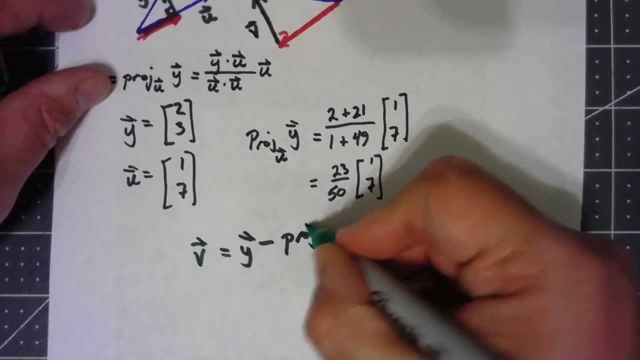 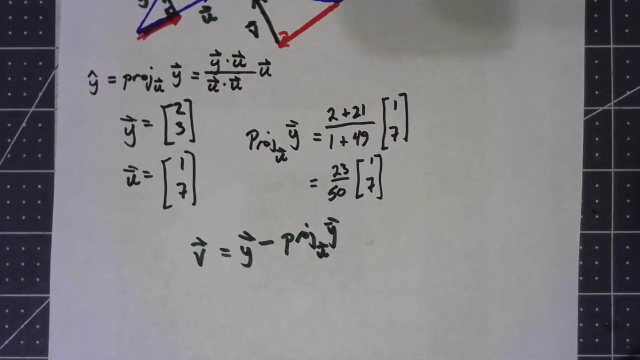 Let's just call it v. If I want to figure out v, I can just take my y vector minus my projection of y onto u, and that's it Again. that's just some simple arithmetic. I'm not going to bother here. 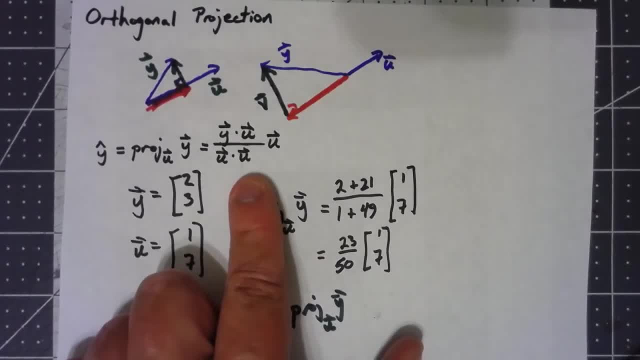 One last thing about this. In the last video I talked about how, if we had an orthonormal basis, we could find our coefficients with respect to that basis just by taking a dot product. Really, the reason that works is this formula. 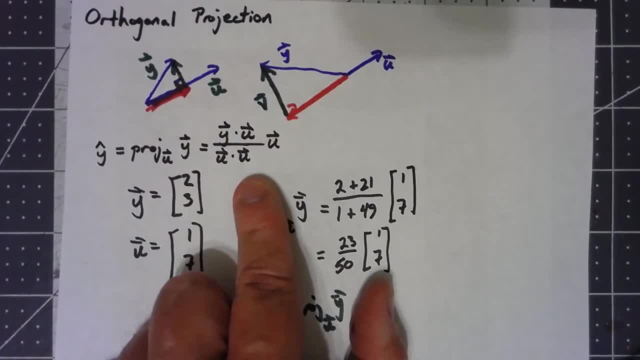 because for any orthogonal basis the coordinates are just these coefficients. in this projection It's the y dot u over the u dot u. But because we had an orthonormal basis- u dot u- the magnitude of the vector squared is 1..